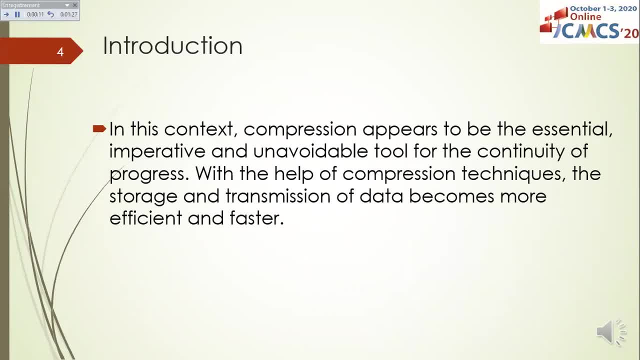 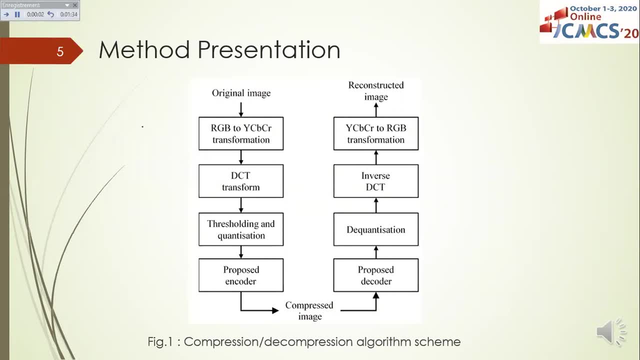 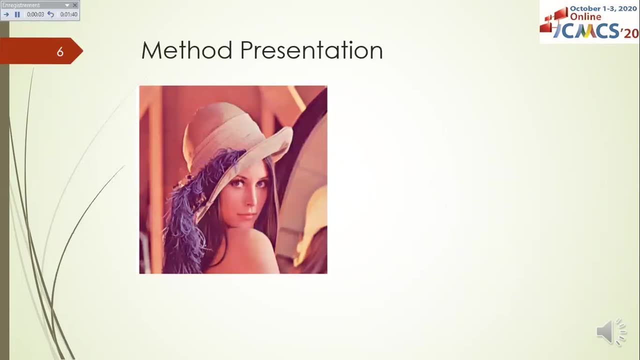 This helps to determine the continuity of the progress. With the help of compression techniques, the storage and the transmission of data become more efficient and faster. This figure represents the compression decont. After the space color transformation and in order to perform the DCT, the image should: 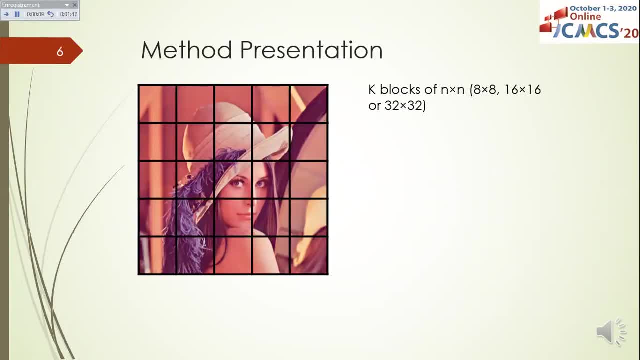 be divided into cubed blocks and DCT transforms as applied to all blocks of the image. The DCT inequality shifts as the system candy transitions. It makes sense for the partnership between the two systems. The merged images do not allow for wear and tear, only left hand which is pickup some patients, Juliana. 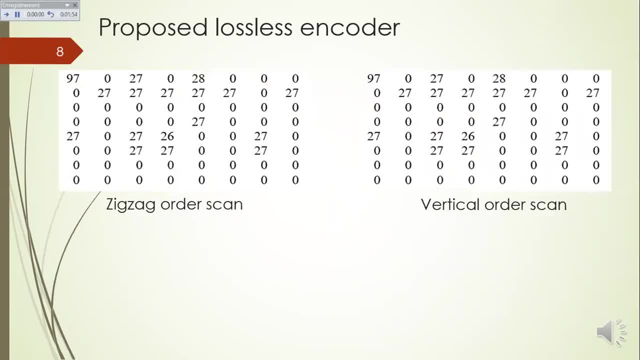 The DCT blocks are quantized and thresholded. The well-known differential DC encoding is used to encode the DC coefficients. To encode the rest of the block, the proposed encoder uses two scan orders, namely zigzag and vertical, for reading the DCT blocks. 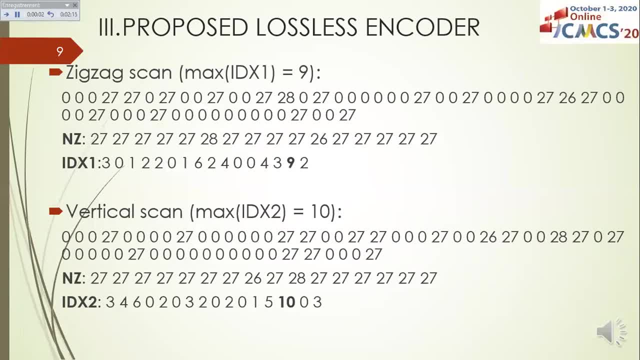 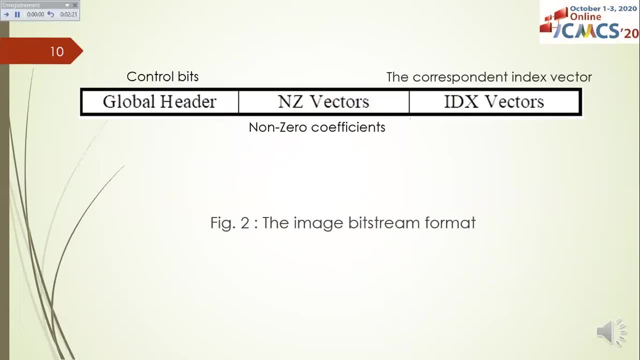 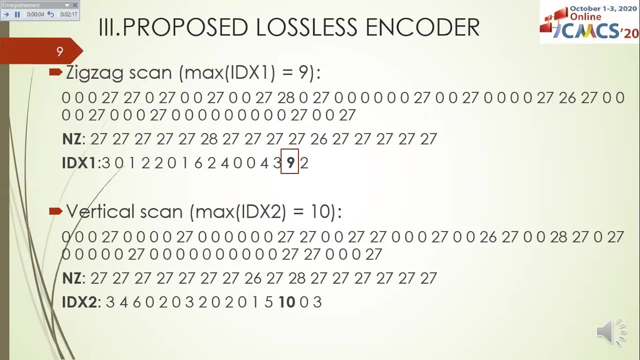 The resulting vectors are: the bolded values are the maximum values of indexed vectors. The smallest value of these maximums is 9.. Thus, for this block, the best scan is the zigzag scan order. The encoded image, bitstream, is shown in this video. 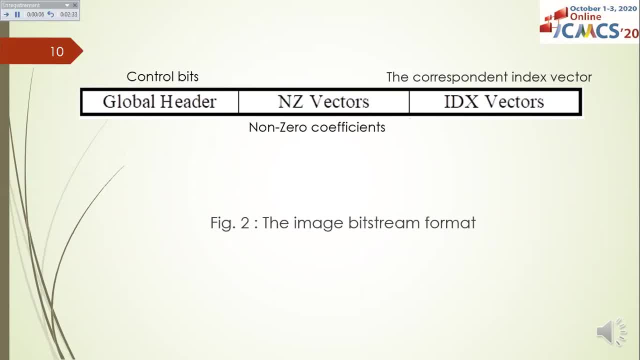 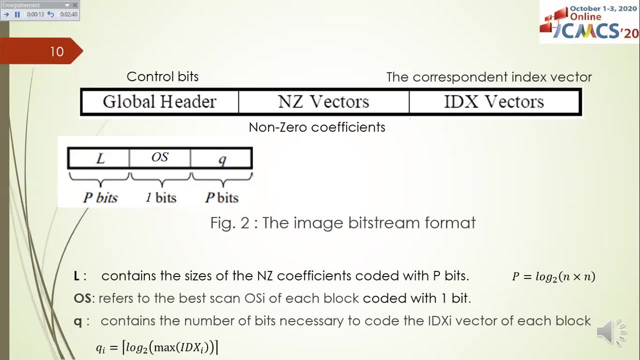 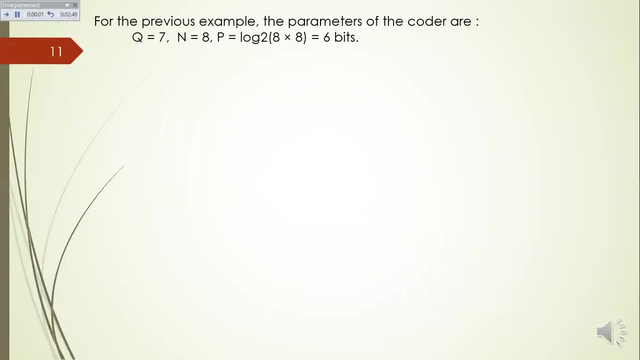 And it is composed of a global header containing control bits and two other vectors. The global header is composed of three parts: L, OS and Q. For the previous example, the parameters of the encoder are and the bitstream is the number of bits needed to encode this block is. 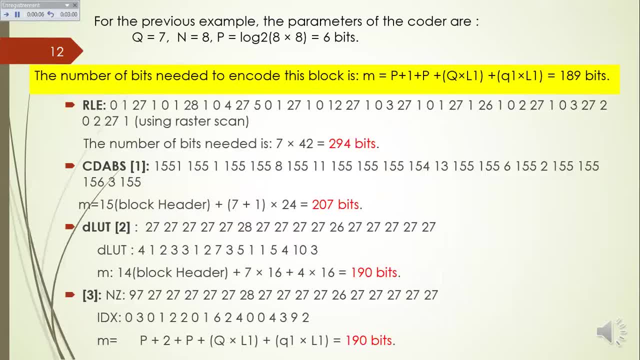 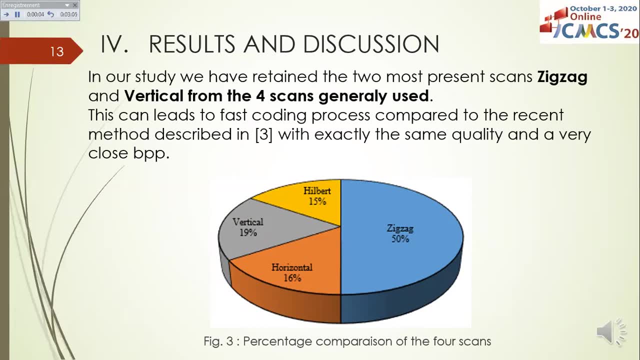 and nearly similar methods for the scan order. The encoded image bitstream is the number of bits needed to encode this block is The same blocks gives. In our study we have retained the two most present scans- zigzag and vertical- from the four scans generally used.